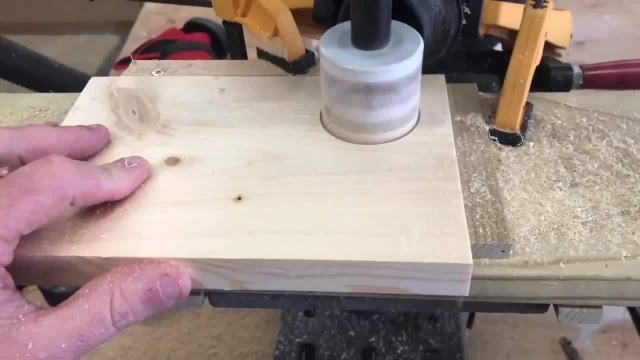 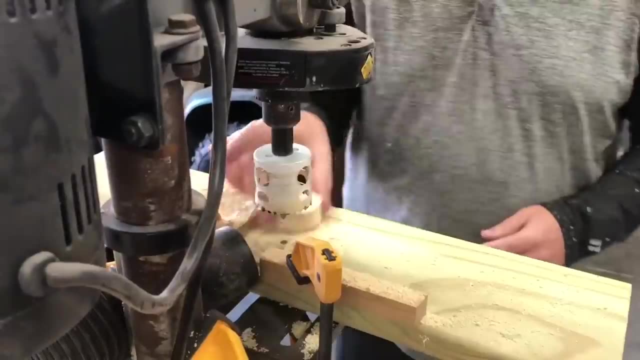 And I usually start with the front and the middle first to work on, And each one of those gets a hole that's about an inch and a half drilled in the corner And I have a jig set up on my drill press that cuts out these little circles. 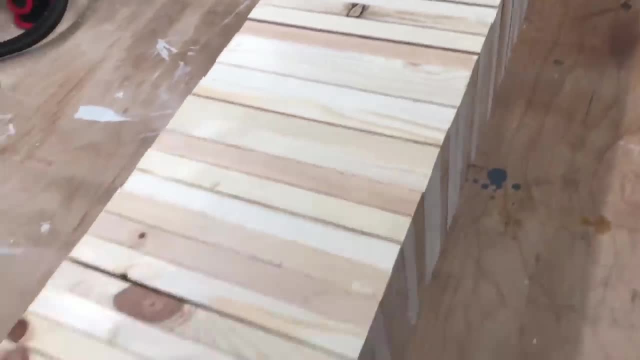 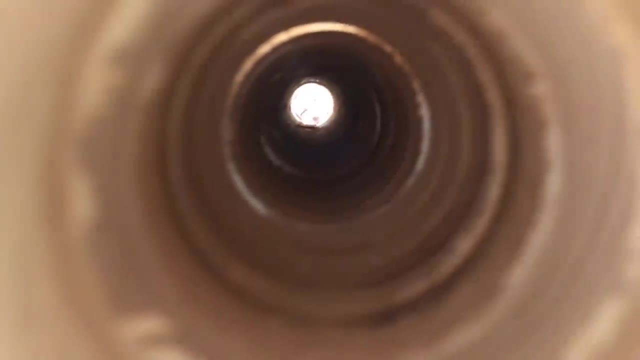 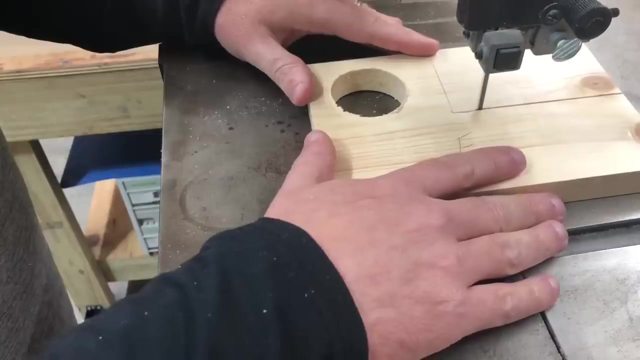 So if anybody has any idea what to do with these little circles, make a comment down here. make a comment down below, please, because I have tons of those things. After that is done, I take them over to the bandsaw, cut out the corner pieces of the front. 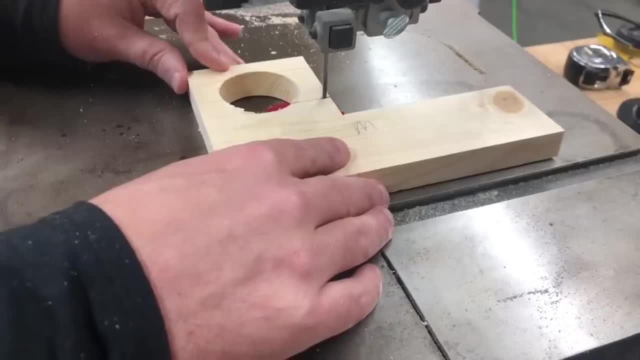 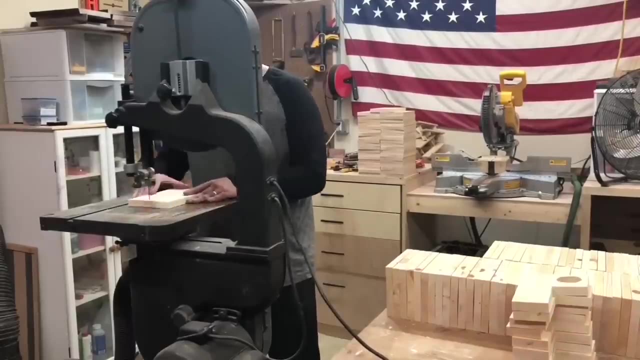 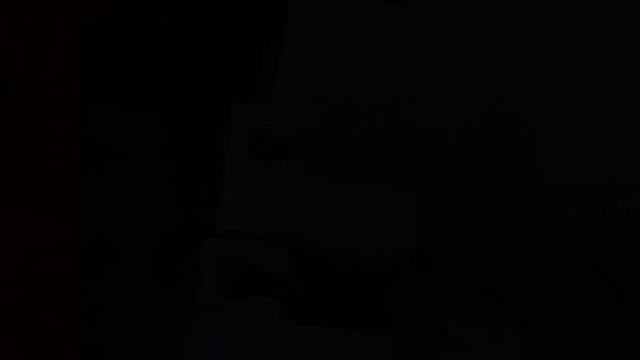 and the middle. Now the middle piece is sandwiched between the front and the back and that gets a notch cut out of the hole. Then, once those are done, you lay them out and I sand them now just to make it easier to. 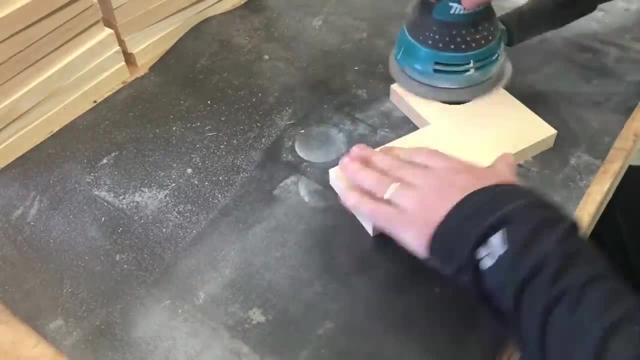 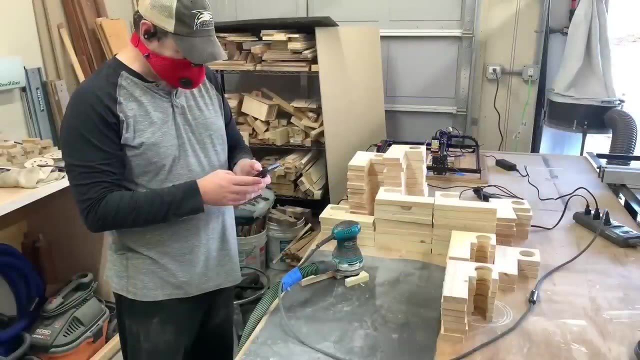 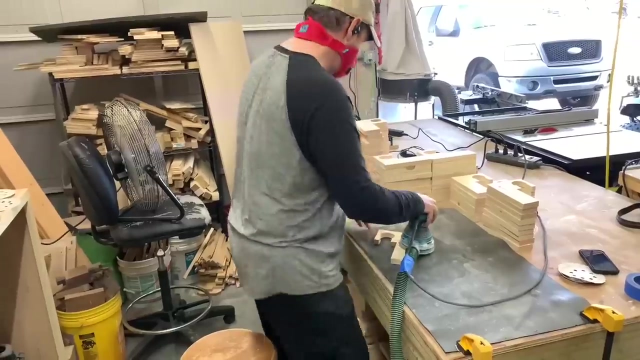 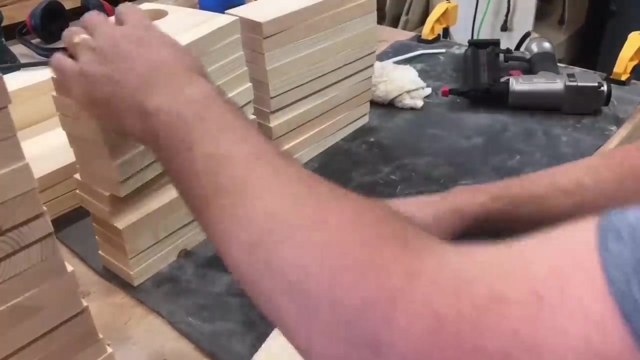 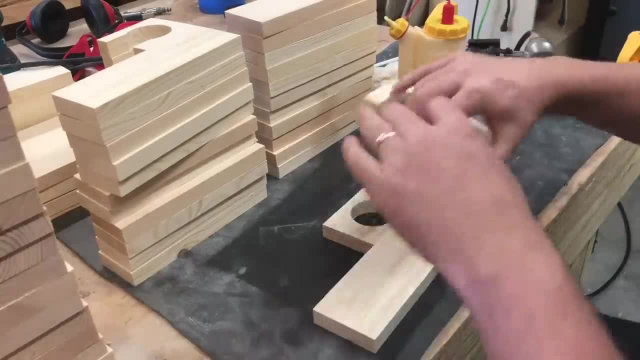 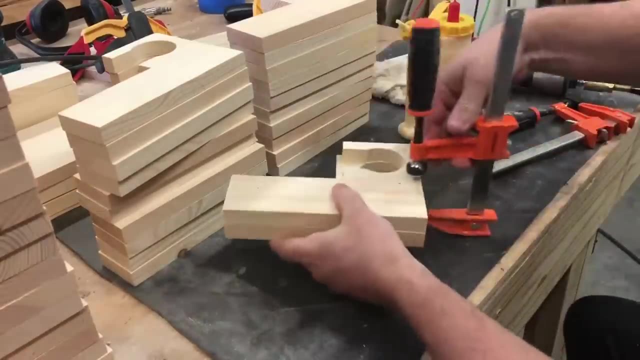 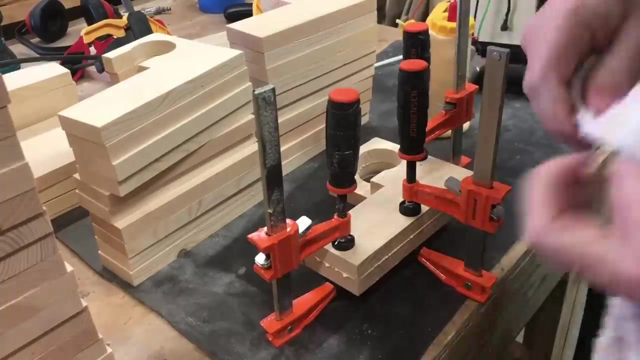 first I'm using a fancy glue spreader, but because there's so much in there and these things tend to slide around, I do drive a one-inch brad nail in there a couple of spots, just to hold it, so that I can clamp these up and get them to really seal up the front and that center seam. 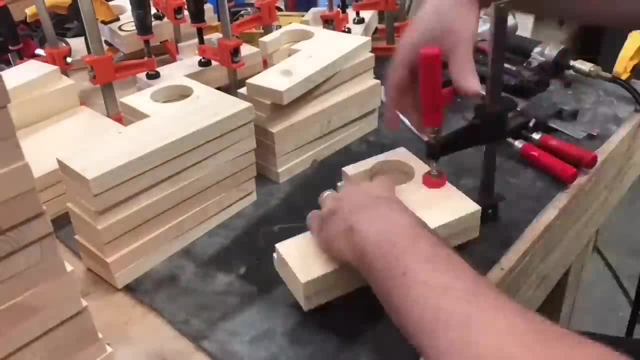 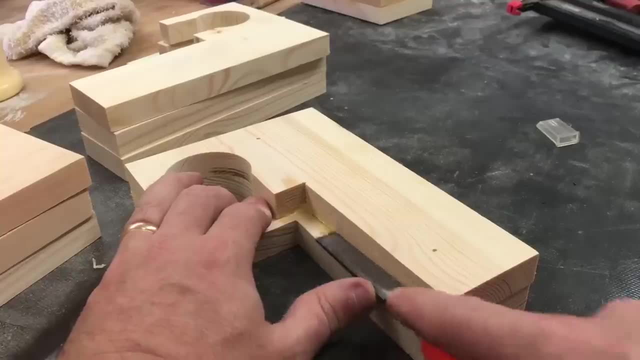 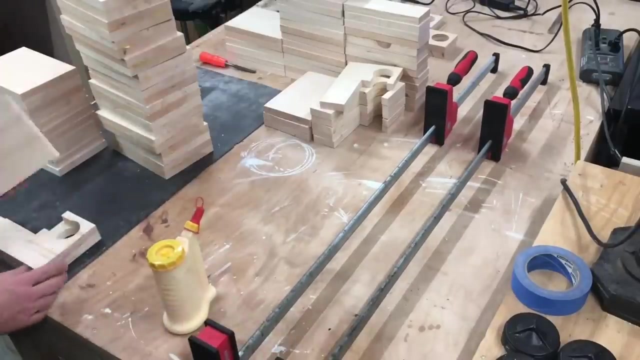 And then the hardest part of this thing to sand is that hole. It's the best time now to sand those. While you've got just the front, you can get access in there. The next step is to glue on the back, and once you glue on the back it kind of closes up that hole. 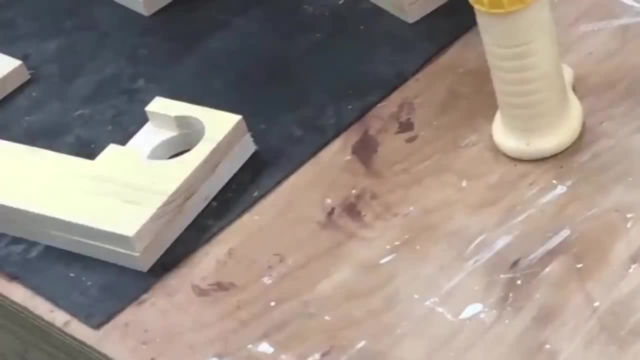 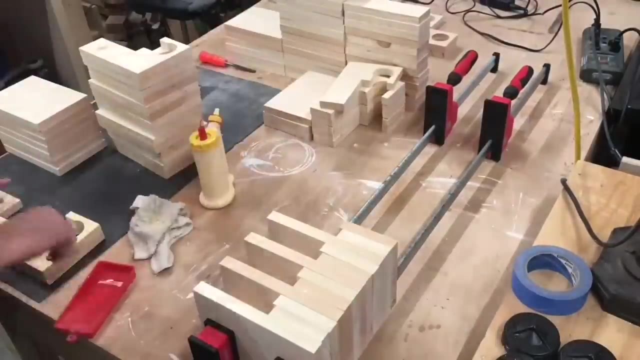 Again with the fancy glue spreader you spread it. get that back piece lined up. then I like to stack them multiple deep, because this is many of these being built- Low clamps and clamp them up tight. You got to seal up those seams. 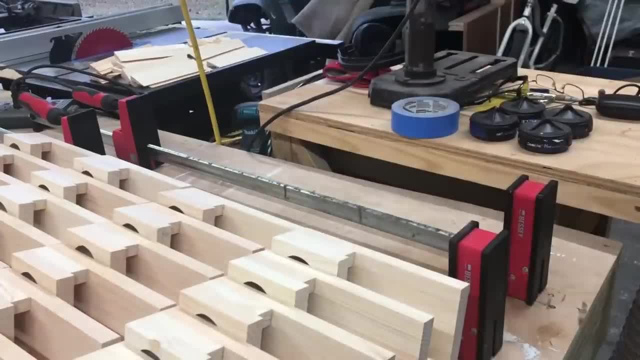 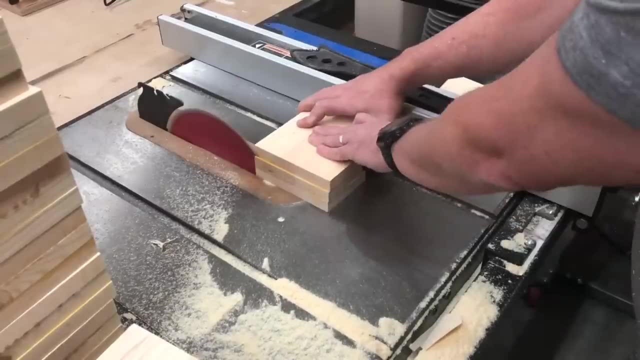 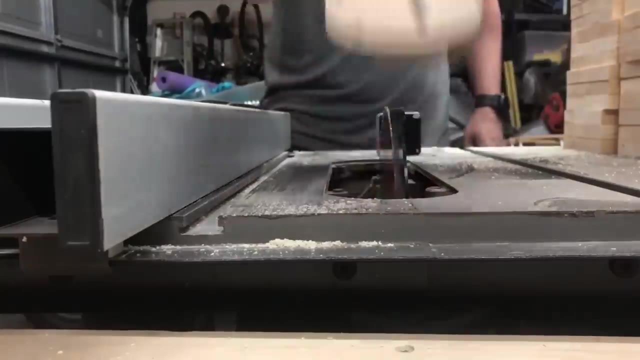 Take them out of the clamps and then I usually run them through the table saw just to kind of clean up the edges a little bit. It does knock off that glue, squeeze out, but it does even everything up, even if they slide around. And then on the bottom I like to put a 15 degree bevel on that thing. so 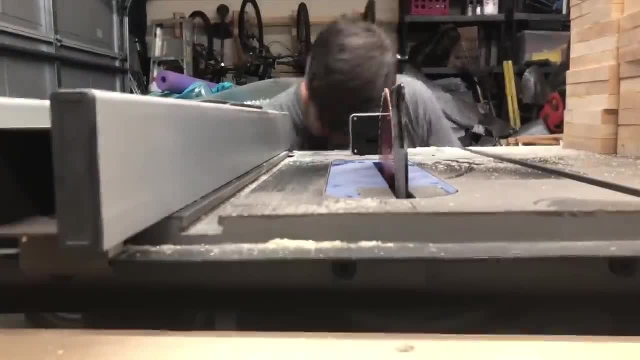 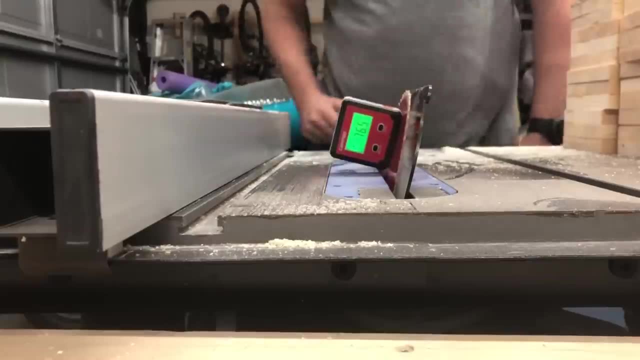 that it kind of tilts back a little bit when you set your cell phone in there. You don't want your cell phone falling out. So I've found out that that 15 degree bevel is a perfect angle to allow that thing to lean back and then also not fall over very easily. But inevitably, some of these 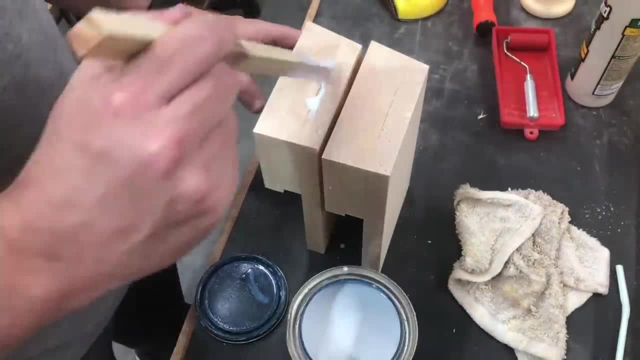 boards, especially these pine, like to twist and bow a little bit, so there's always a gap here or there, But it's not a problem. And then I like to put a 15 degree bevel on that thing so that it tilts back a little bit when you set your cell phone in there. You don't want your cell phone falling out. 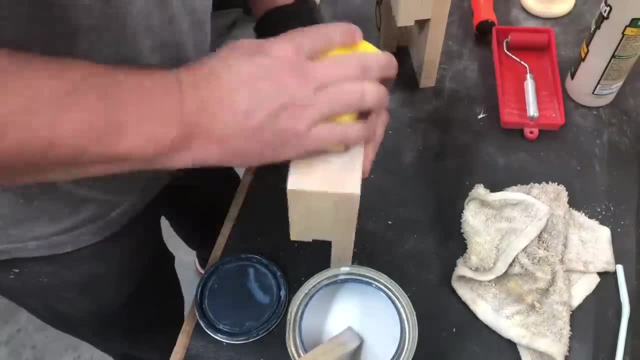 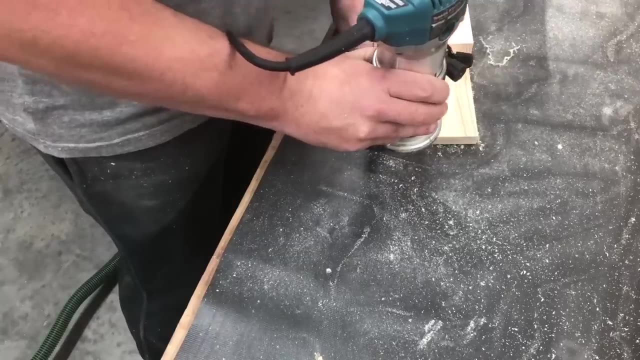 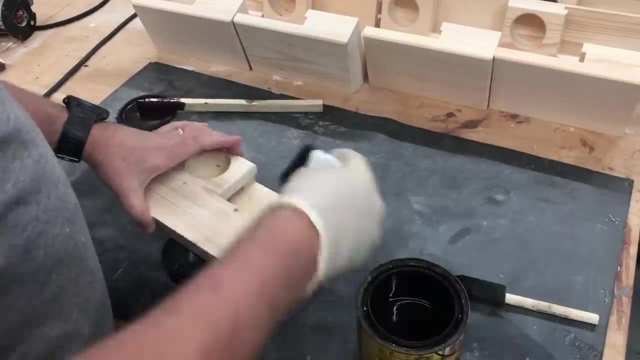 But I feel like I just put poly on there and sanded it in Ground off the edges with the quarter inch round over bit. That softens those edges a little bit. Once it's all done, I usually spread stain on them. For these things I use honey, Like that's one of my favorites. 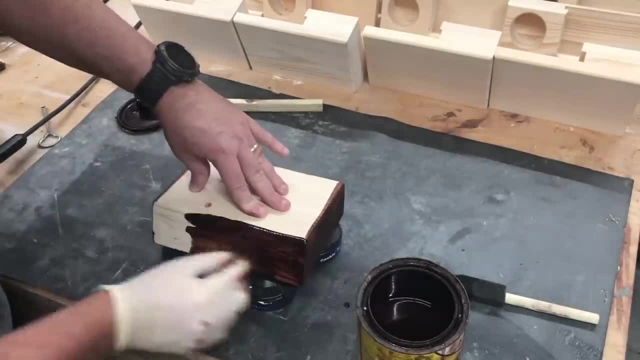 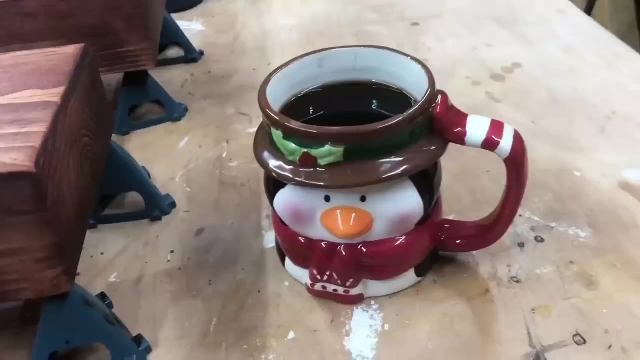 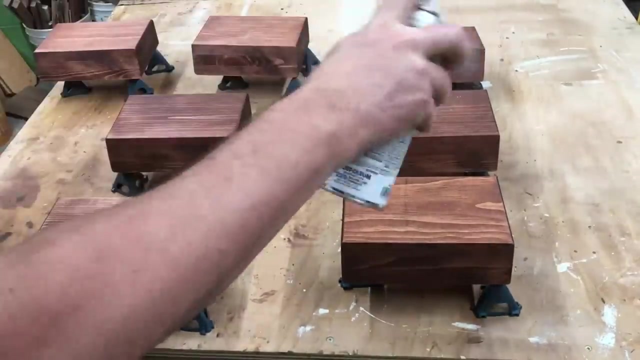 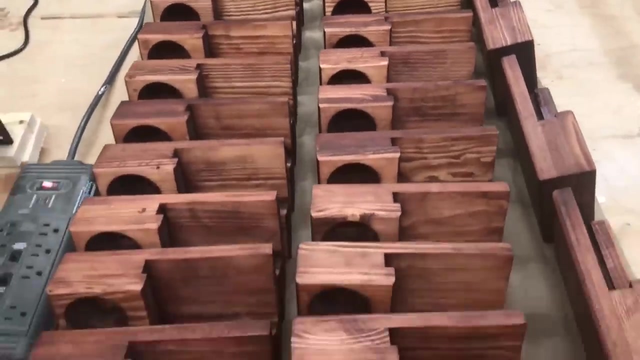 Once that's dried up, you spray on the polyurethane and that covers it in about two coats. Now these actually have a laser engraved logo on the front of them because they were corporate Christmas gifts. So I'm just going to put a little bit of that on there And then I'm just going to 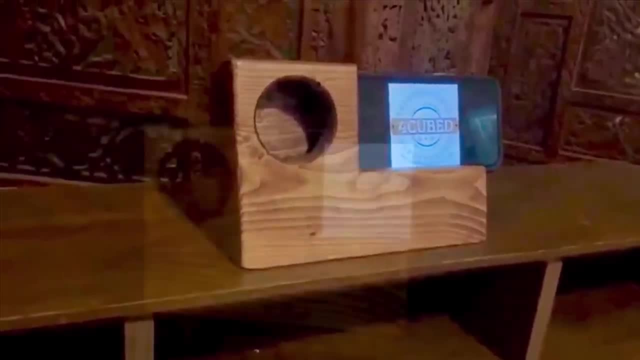 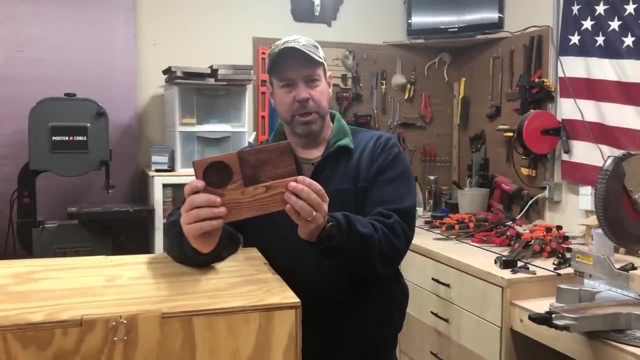 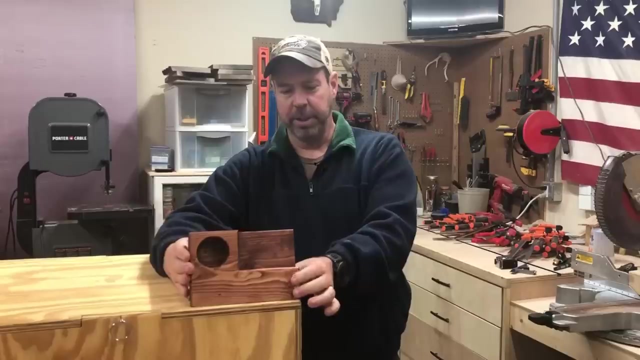 put a little bit of that on there, And then I'm just going to put a little bit of that on there. So this little thing has been a little surprise for me, because over the last probably two years since I've been making and selling these, I've probably sold maybe 50 or more of these things. 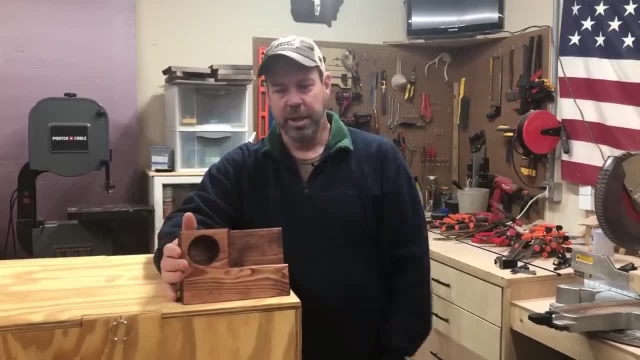 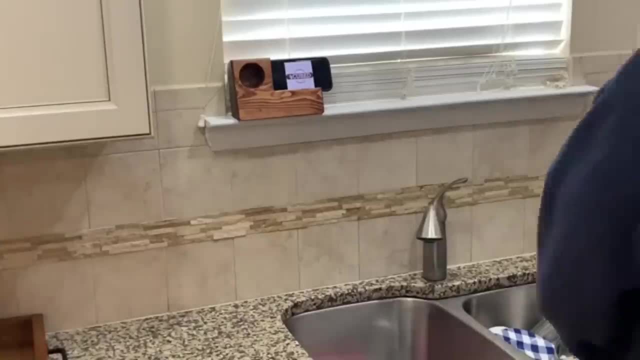 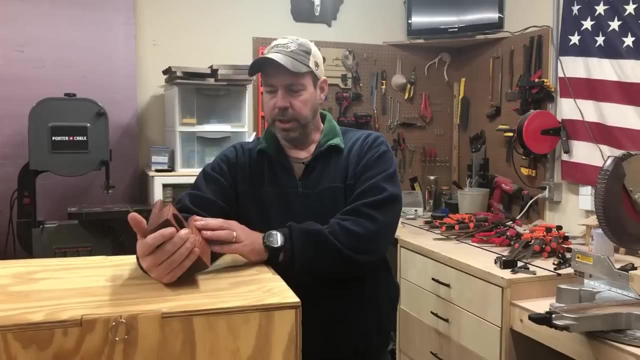